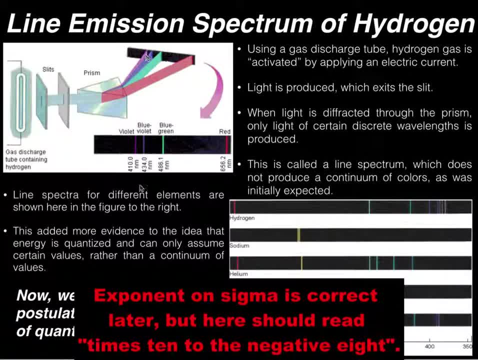 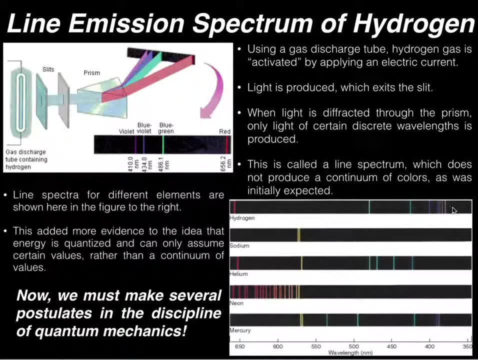 current. the light is emitted, it goes through the prism. you only see a few marks. You see red here. you see blue-green, blue-violet and violet. Here's another look of what they found right here. Here's the hydrogen emission specter. So what you see here is there is not a continuum of values, There's only. 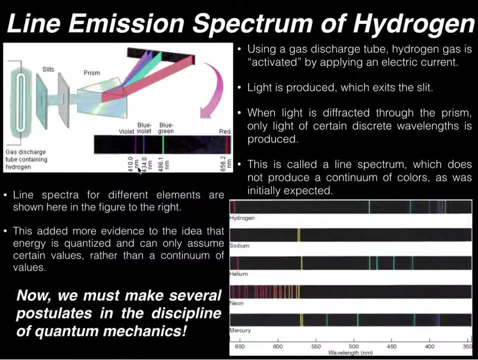 discrete values and that value is given as the nanometers, the wavelength right, But we know that wavelength is related to energy. So basically, what they're saying here is: energy is not a continuum of values. on the quantum level It is quantized. It only takes on discrete values. 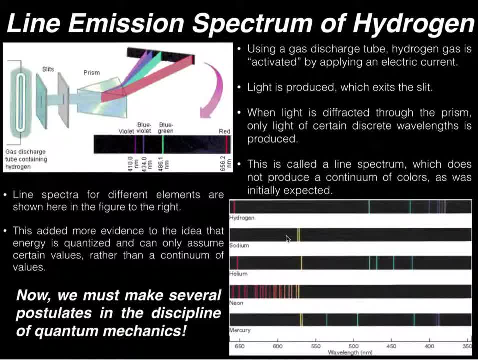 And this experiment was replicated with a bunch of other elements of sodium- not near as complicated, but it's still discrete: Helium, neon, mercury, and so on and so forth. You can do this with any of the elements, And what you'll find is the energy only takes on discrete values- discrete. 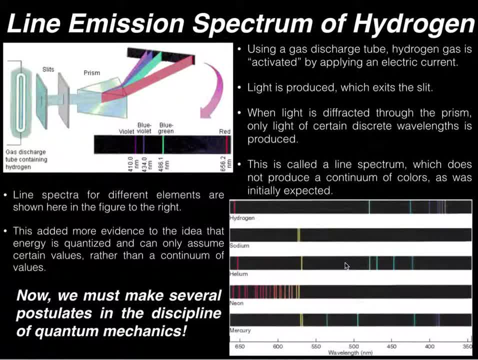 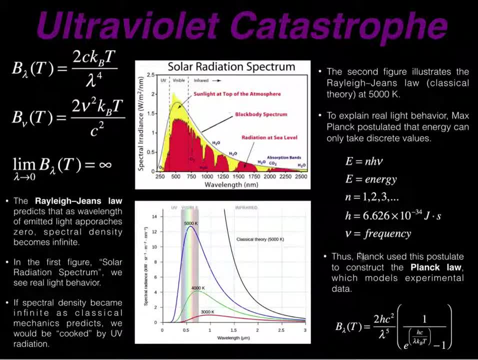 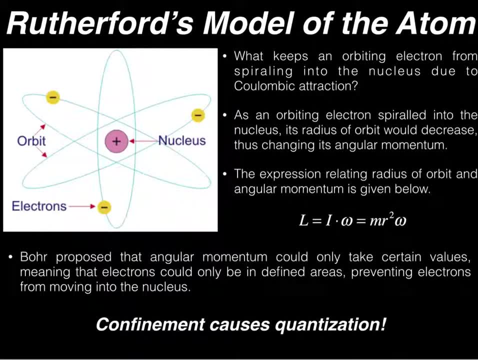 wavelengths, all right, And this along with all the previous experiments, with the ultraviolet catastrophe and black body radiation, with Max Planck, the photoelectric effect, with Albert Einstein, Bohr's correction and postulates about the model of the atom, now with the line emission. 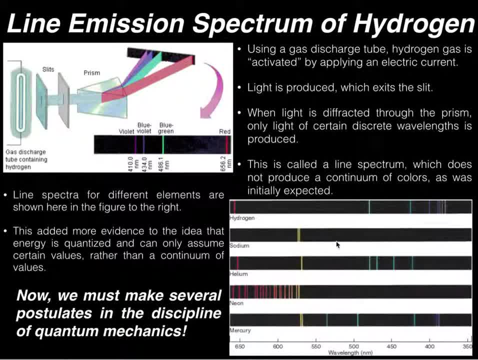 spectrum of hydrogen and these other particles or these other elements. we now know that energy does not take on a continuum of values, and possibly particles like electrons don't either. They take on discrete values of energy, discrete values of angular momentum, And this, at the very turn of the 20th century, initiated the field of quantum mechanics. 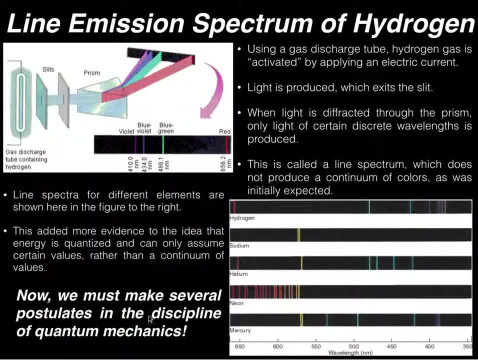 So now we must make several postulates in the discipline of quantum mechanics, And I'm going to end this playlist with this, And so what we're going to do now is switch playlists. So I recommend you go look at the playlist where we talk about the postulates of quantum mechanics, And there's 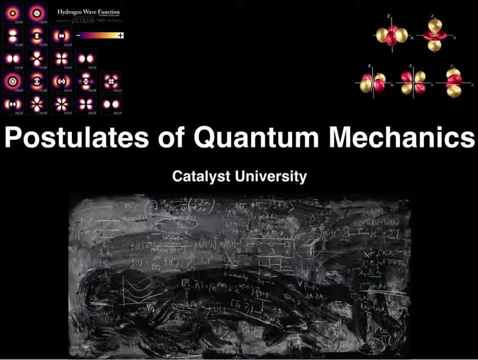 several of them and we'll jump right into the discipline. Thank you for watching this video. Make sure to like it and subscribe.